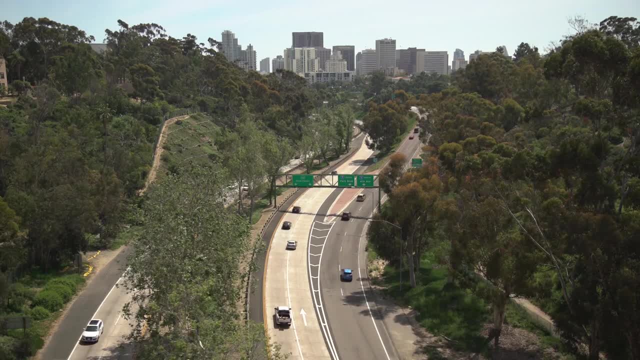 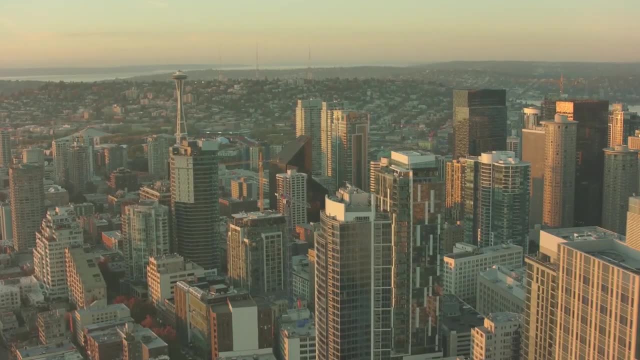 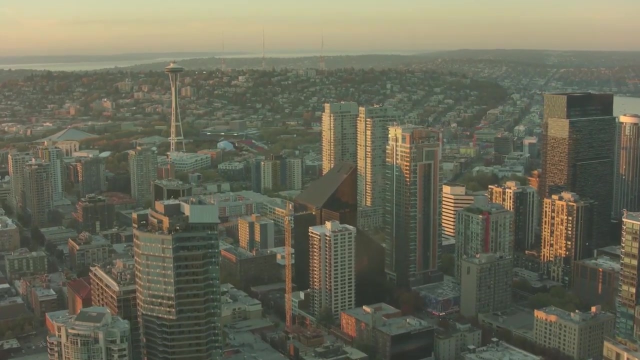 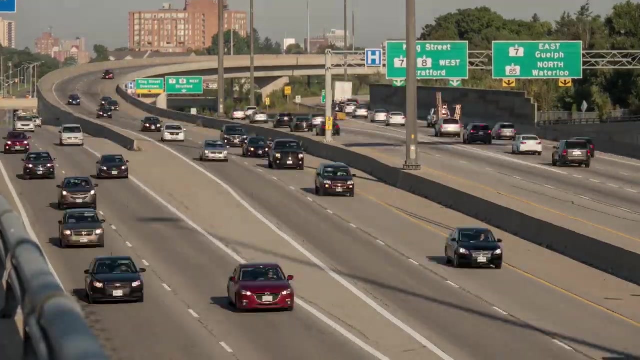 for transportation needs. Urban sprawl is also caused in part by the need to accommodate a rising urban population. However, in many metropolitan areas it results from a desire for increased living space and other residential amenities. Urban sprawl has been correlated with increased energy use, pollution, traffic congestion and a decline in community distinctiveness. 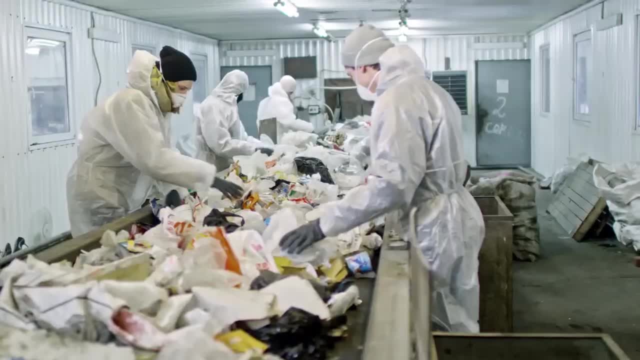 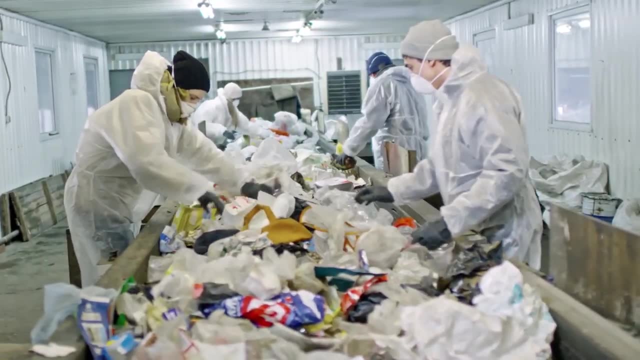 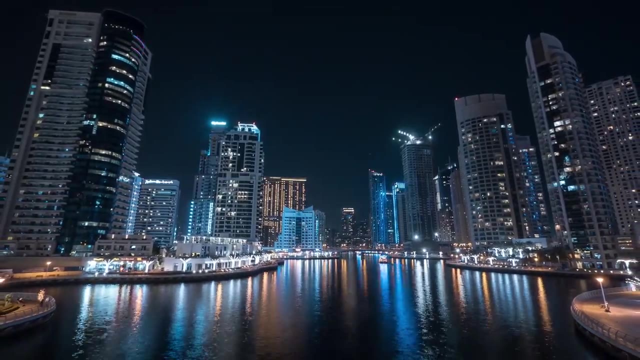 and cohesiveness. In addition, by increasing the physical and environmental footprints of metropolitan areas, urban sprawl is becoming increasingly popular. This leads to the destruction of wildlife habitat and as well as to fragmentation of remaining natural areas. So why does sprawl matter? Well, growth is inevitable in areas where people want. 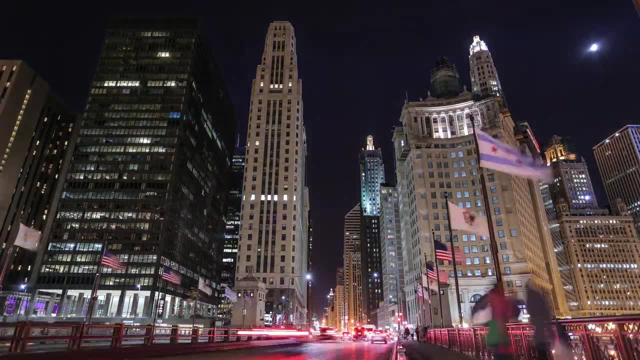 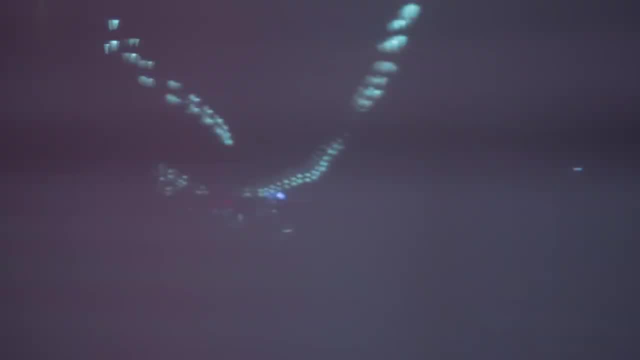 to be and live in, So it's logical for growth to occur and expand outward, or is it? Yes? while sprawl contributes to growth and, more importantly, economic growth, there are many consequences to the growth of urban sprawl, For example, if you want to live in rural areas. 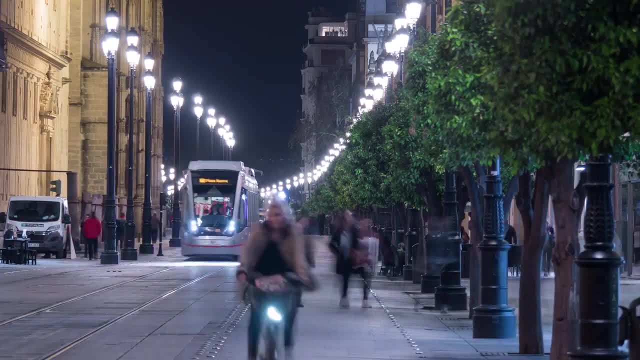 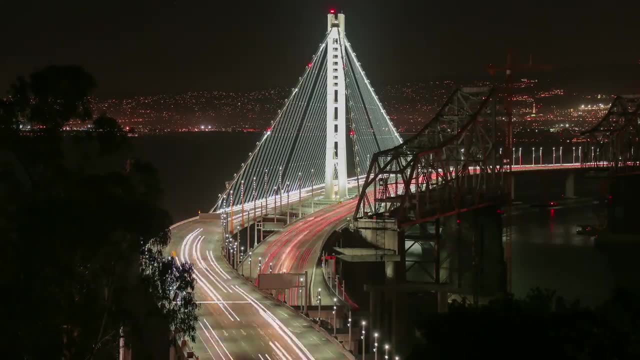 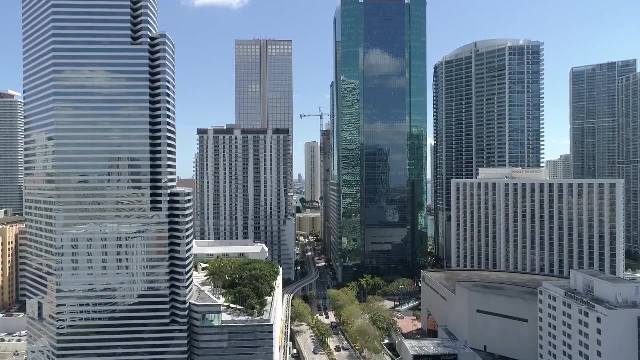 you have to live in rural areas. If you want to live in urban areas, you have to live in rural areas. But are these costs weighted though? Well, let's see. Sprawl means less walking, more driving, more energy consumption, more pavement, more built space. It also means for many people: 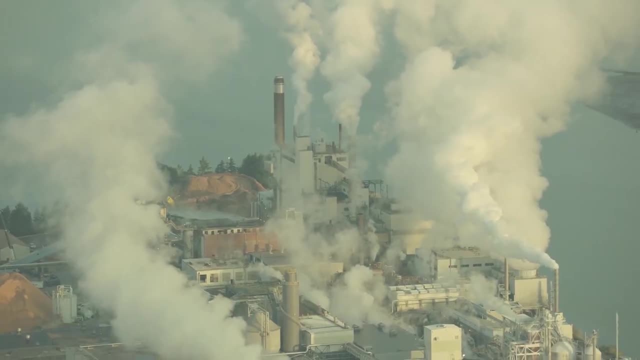 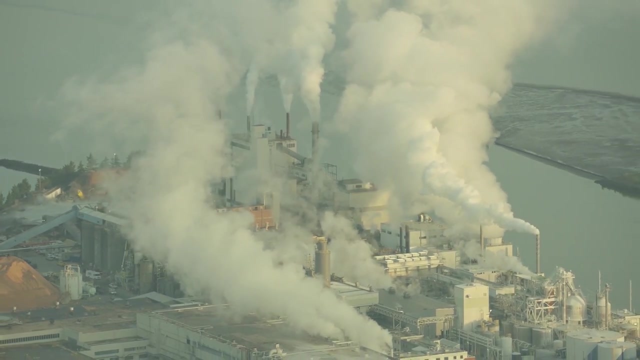 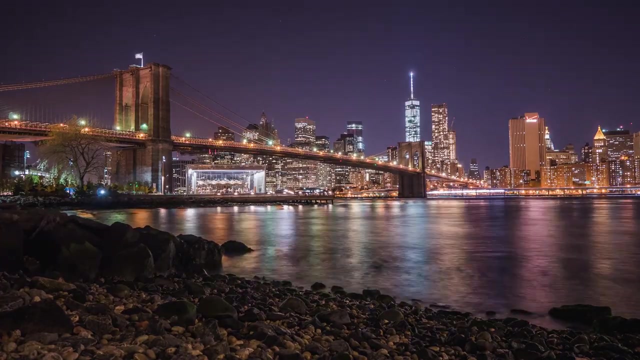 less exercise, more pollution and less green space. This all leads to a worse quality of life eventually. So why is it so ideal? Close to the city, but within commuting distance is very ideal for many More, so the idea is not necessarily to 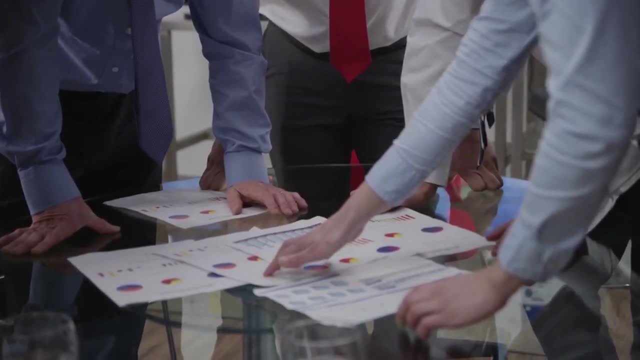 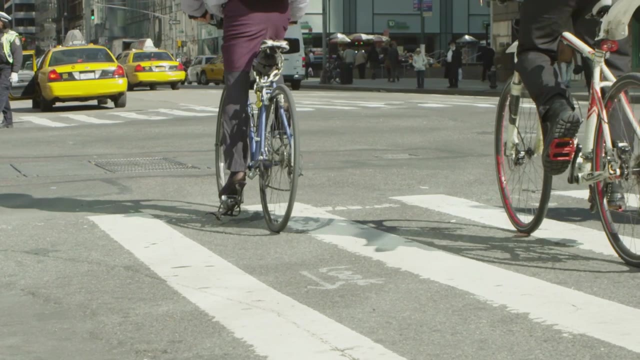 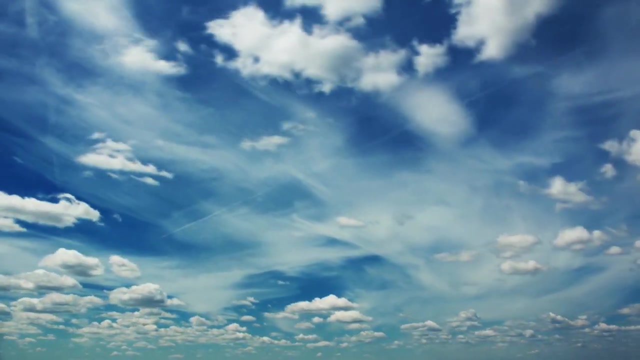 slow sprawl. but, more generally, how do we make existing places better? We're looking at smart growth, well-planned developments that channel growth into existing areas by investing in cities and older suburbs, while preserving space and protecting the environment. This could also mean 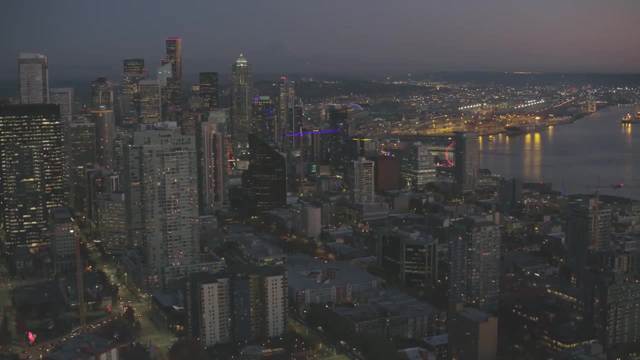 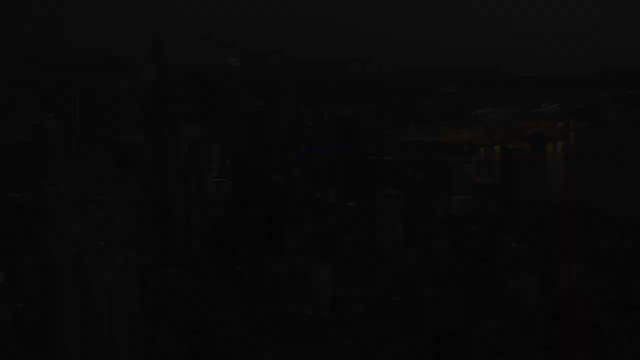 sustainable development, which means that we're going to be able to create more sustainable development, which is society, economy and environment together equally weighted.